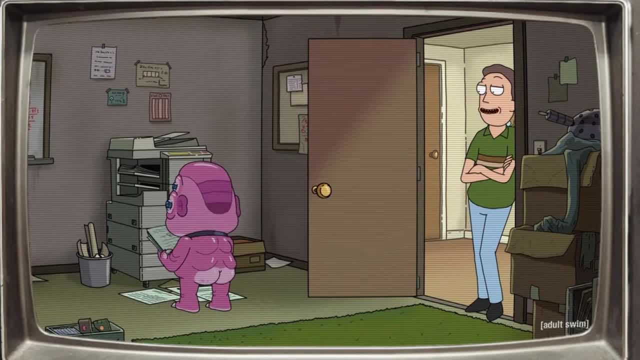 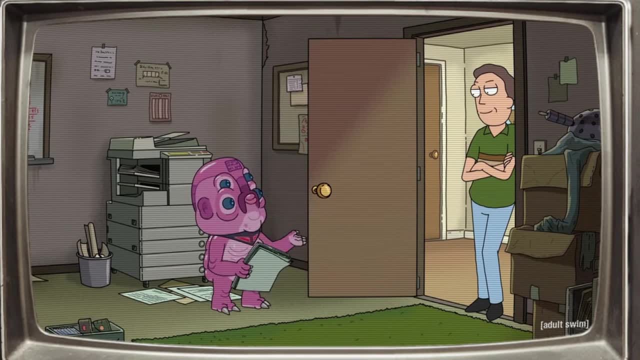 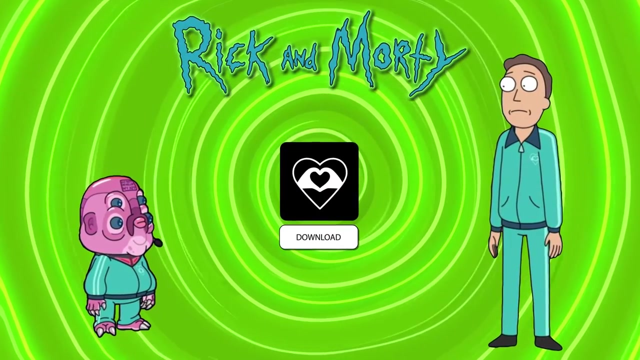 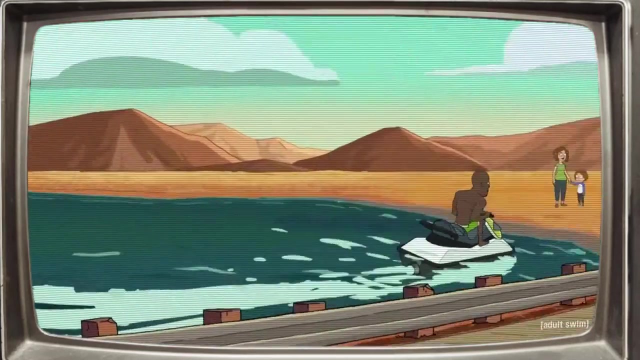 In this episode of Rick and Morty, Jerry falls into a trap by agreeing to develop an app he knows nothing about. The app is launched shortly and the world faces the consequences. This is not something we have to worry about in real life, but the show is parodying an. 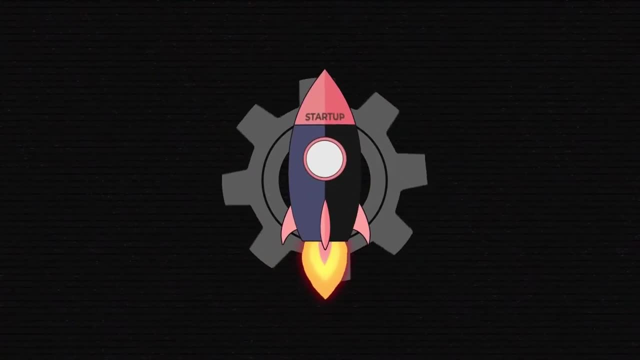 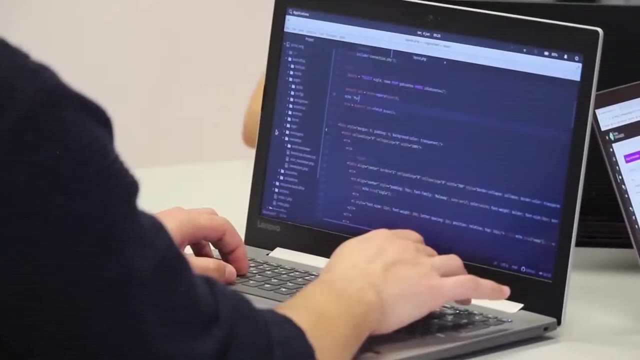 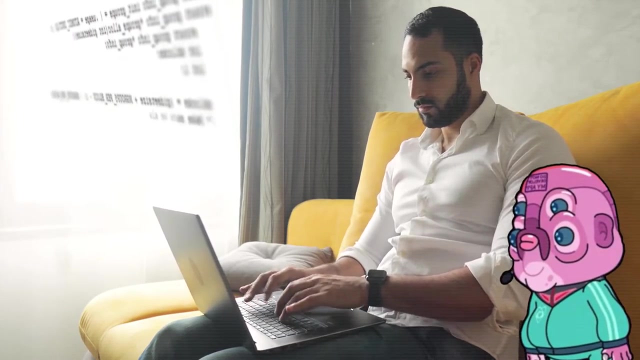 actual startup phenomenon: The culture of hatching new products without much planning or preparation, driven by excitement and the hope for success. Software development is never as easy as on Rick and Morty, since presumably you don't have an alien on the team. It's an expensive, time-consuming and risky endeavor To have. 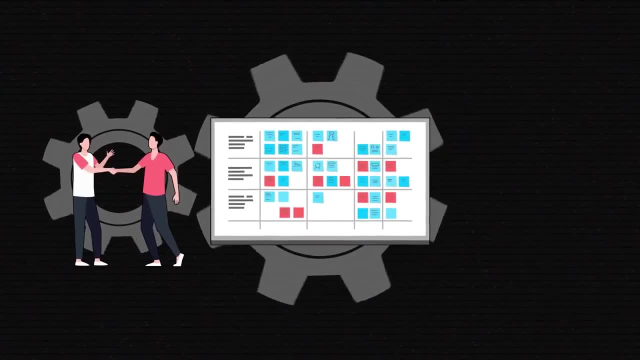 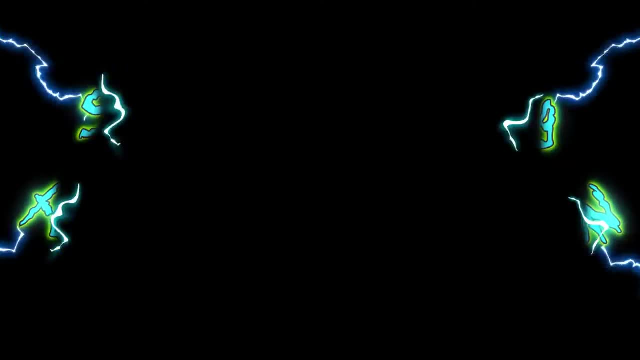 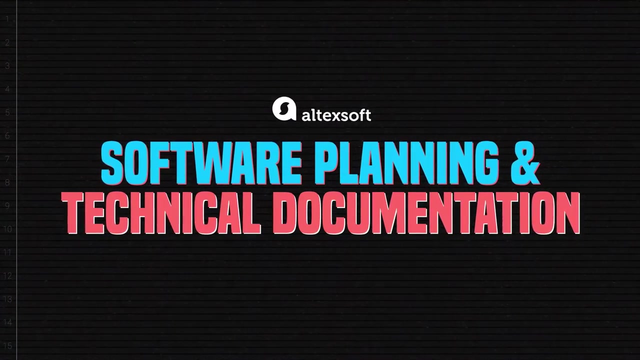 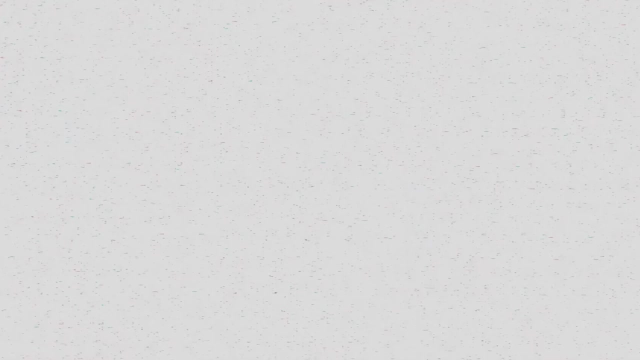 a chance at success. you need clear communication, elaborate planning and documented knowledge and expected expectations. How does this planning happen and what helps devs stay on course? Let's talk about software planning and technical documentation. Luckily, if you're building software, you're not the first one to do that, And even if 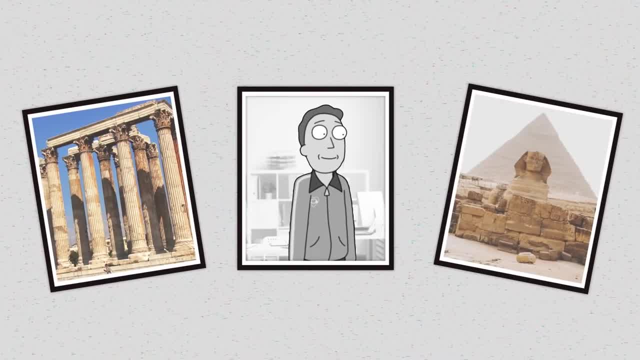 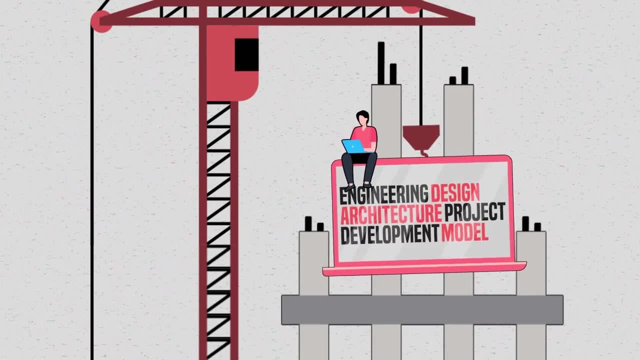 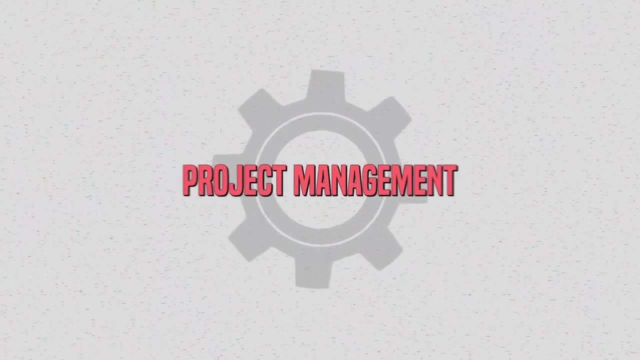 you were, you wouldn't be the first one to build… something. There are many parallels between software development and construction, reflected not only in the wording but also in methods. Project management itself, until very recently, was a discipline associated with civil engineering and manufacturing. That's why, in continuation of the practice, 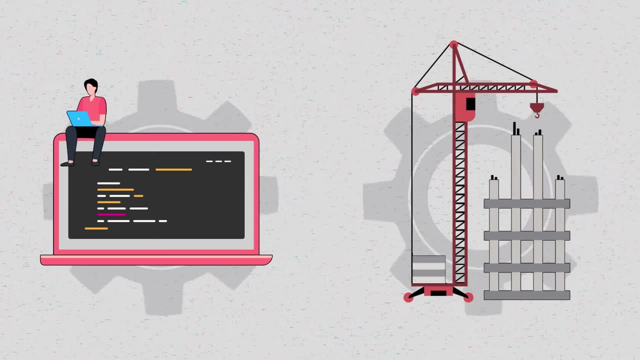 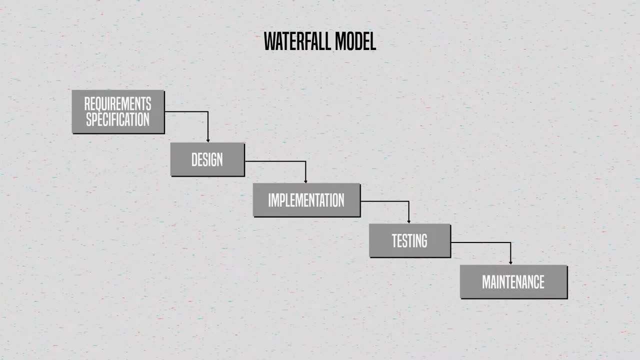 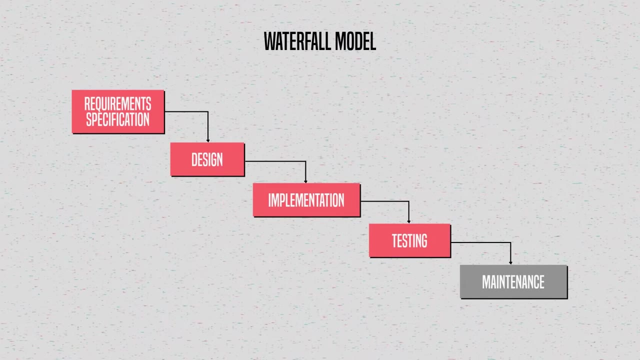 for many decades, software products were built like tangible ones. Look at the now-discredited waterfall model. According to it, the project should follow a few consecutive steps: gathering product requirements, preparing the design, then implementing said design, doing some testing and finally performing maintenance and system support. 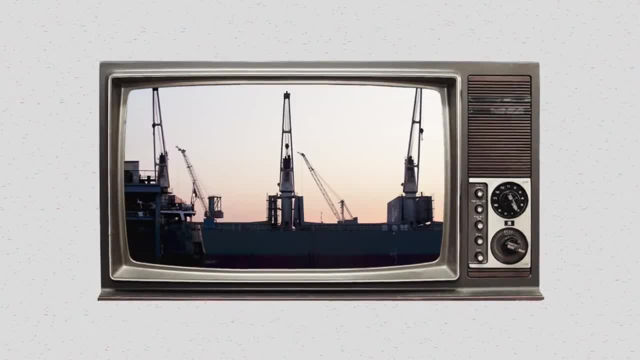 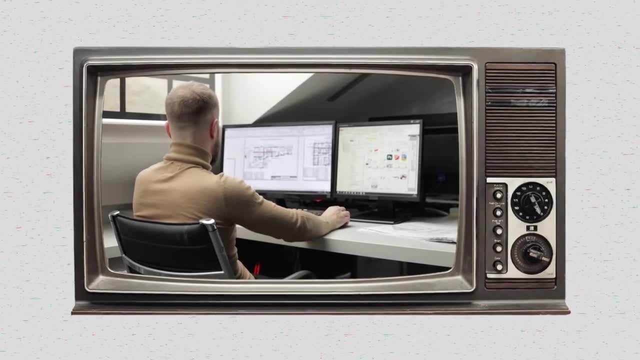 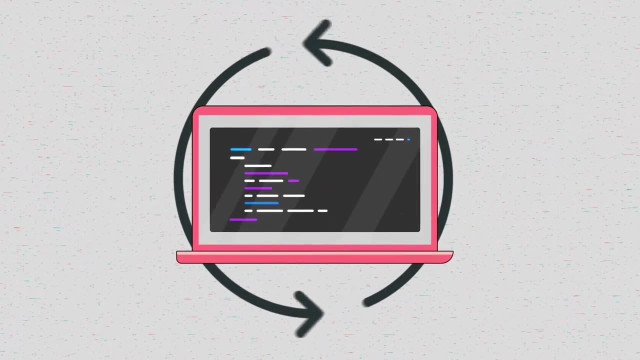 This approach seemed logical because software was treated like buildings or ships or any big construction projects, where you do massive amounts of work first and then apply changes where needed. This, of course, led to failed deadlines, overgrown teams and thousands of lines of code rewritten over and over again Only very recently- 20 years ago, to be more. exact this thinking had begun. The idea was to create a new system, a new system for the project and a new model for the project. The idea was to create a new system, a new model for the project. The idea was to create a new system, a new model for the project. 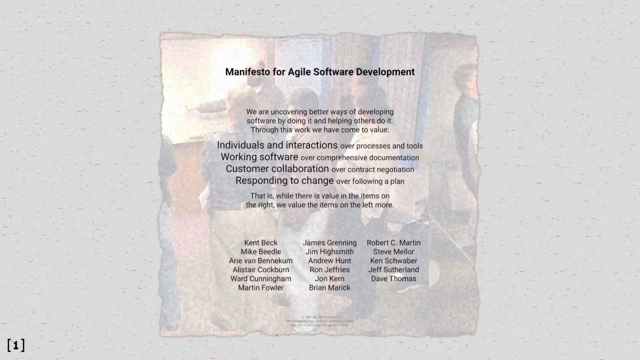 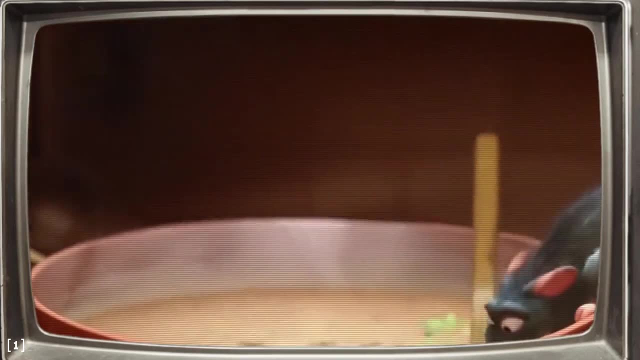 The idea was to create a new system, a new model for the project. The Agile Manifesto questioned the traditional approach and brought the new idea. Building software is an ongoing endeavor where planning should happen along with execution and testing. Today, we enjoy how the Agile principles help us lower risk and always have the ability. 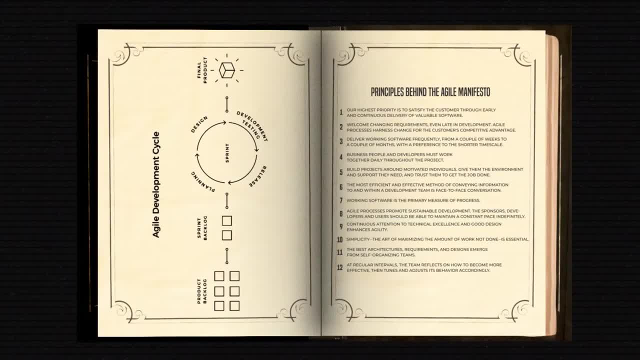 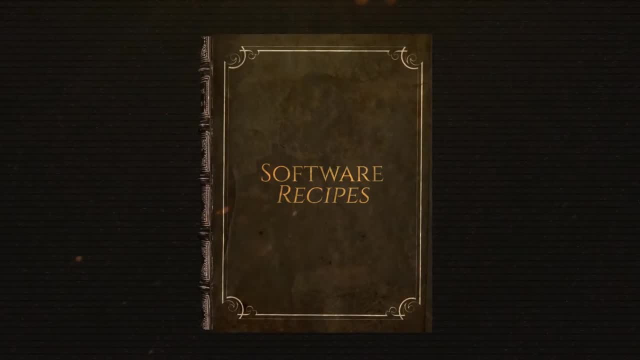 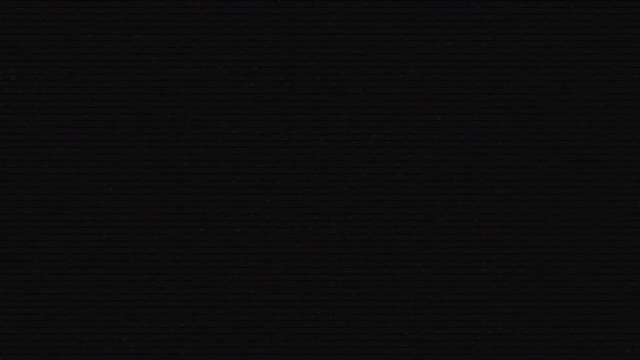 to change something if needed. This is mostly accomplished thanks to great documentation which, just like any other element of Agile project management, is subject to change through operations as needed. So what documents are used in software planning? Software planning is in many ways synonymous with software documentation, because technical 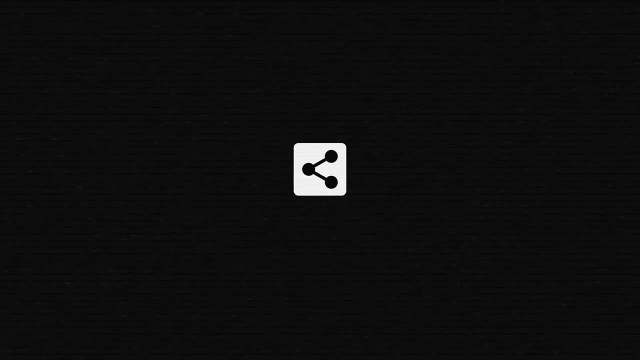 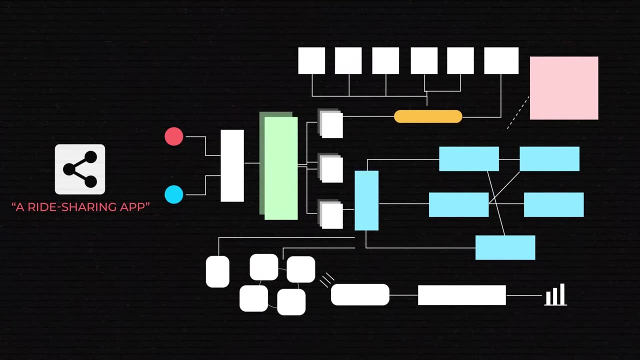 docs is where software starts taking shape. It's where the idea of a ride-sharing app becomes a complex system with its business logic, tech specifications and user flows, and where we first determine the path to this transformation. Ultimately, docs help us answer. 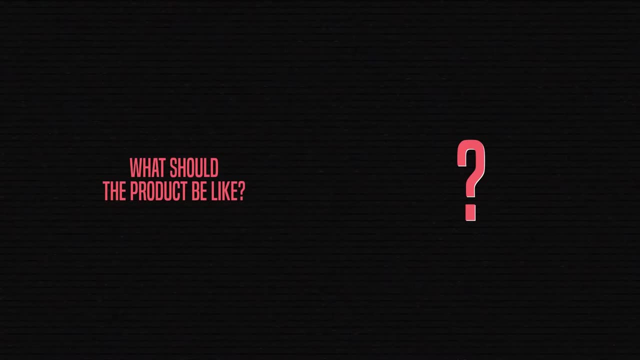 two big questions: 1. What documents are used in software planning. 2. What documents are used in software planning. 3. What documents are used in software planning. 4. What documents are used in software planning. First, what should the product be like? This part of project management is described. 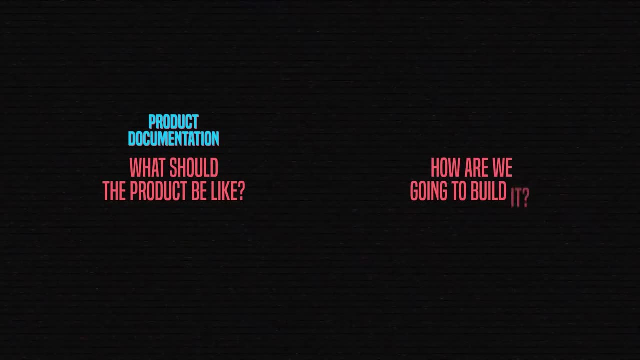 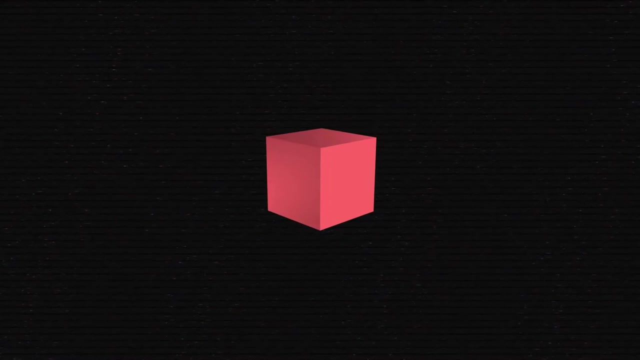 in product documentation. The second question is: how are we going to build this product? It's covered in process documentation. Strap in as we dive deeper into both these groups and we'll start with the what question. A product is a system with a set of features that helps users achieve their goals In software. 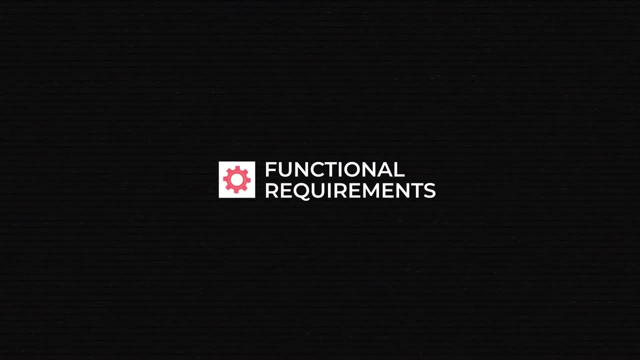 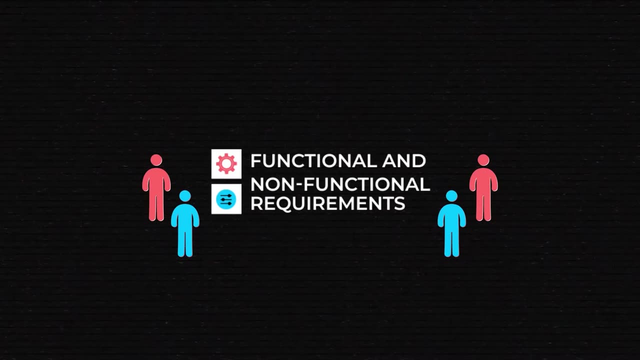 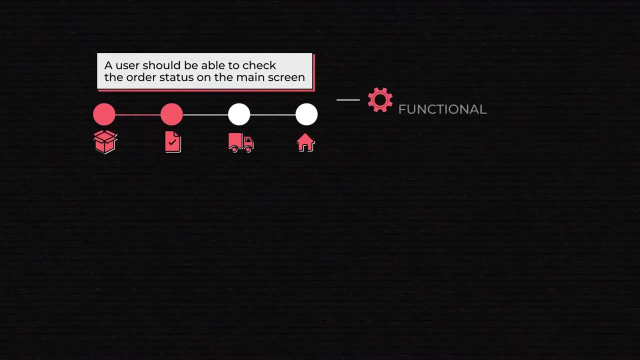 development. these features are called functional requirements, And the properties this system should have are the non-functional requirements. Both are expected by a stakeholder or an end-user to fulfill the product's main purpose. A user should be able to check the order status on the main screen is a functional requirement. 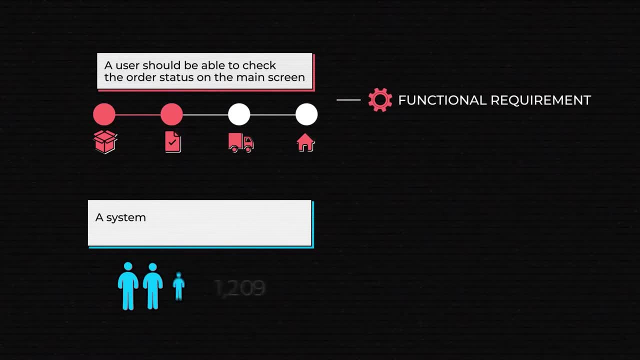 that talks about user capabilities. A system must support 100,000 users at the same time is a non-functional requirement because it describes the capabilities of the product, how fast it is, what security measures it uses. A user must be able to understand the requirements of the product, how the system must grow. 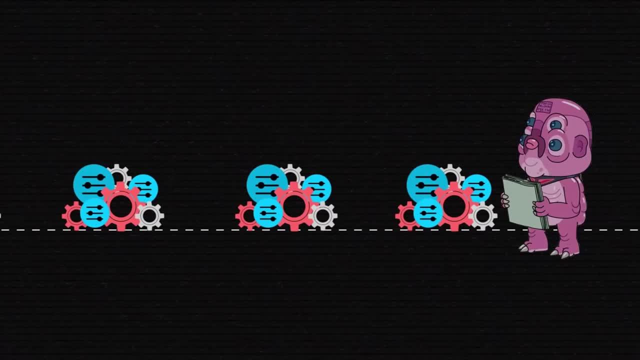 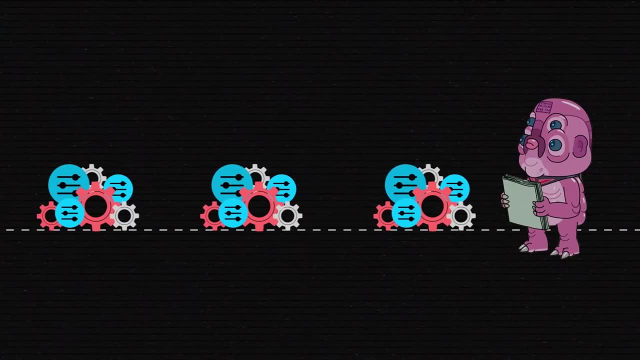 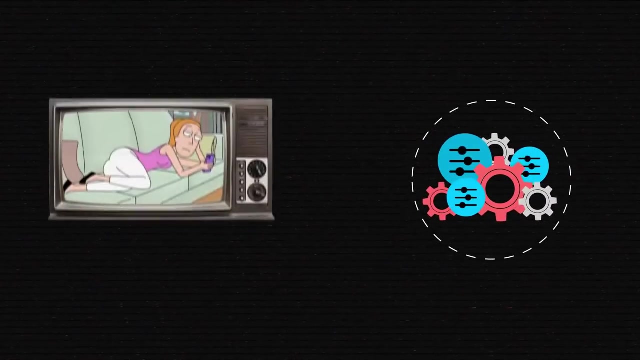 Such concise statements translate user and stakeholder desires into requirements that developers understand and can then plan to implement. A product requirement document is one of the first created. Requirements are largely dictated by users. They're basically the result of all the user research done earlier, when the team talked to real-life people and learned about their 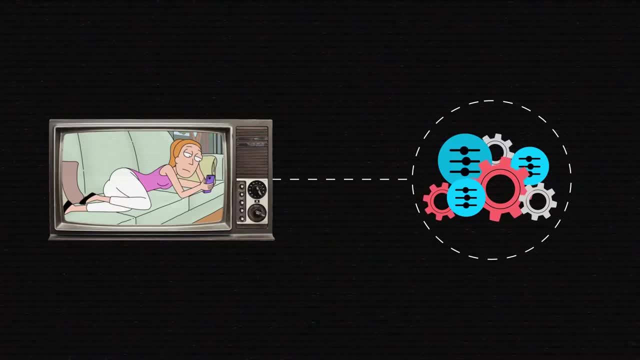 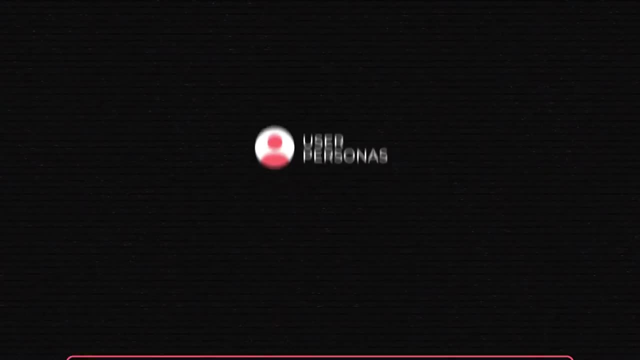 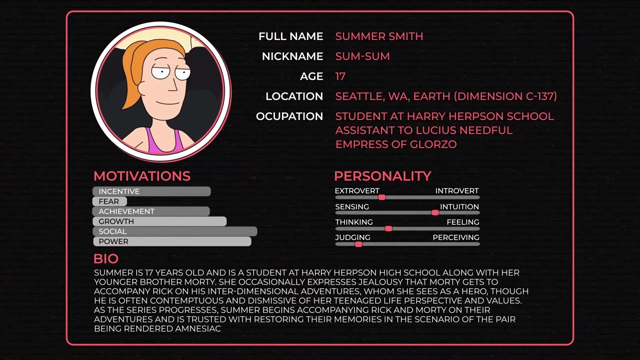 preferences and experiences. This research, though, results not only in the feature list, but in other invaluable pieces of information, For example, in user personas. a persona is a detailed description of a typical user that makes it easier for the dev team to visualize what the people want, need and how they behave. 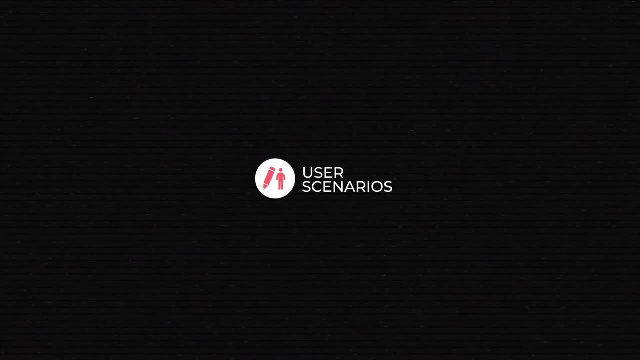 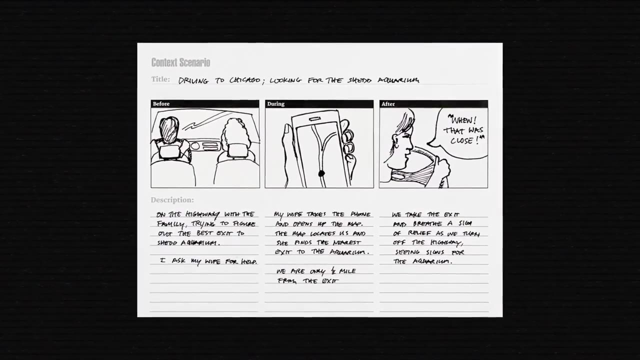 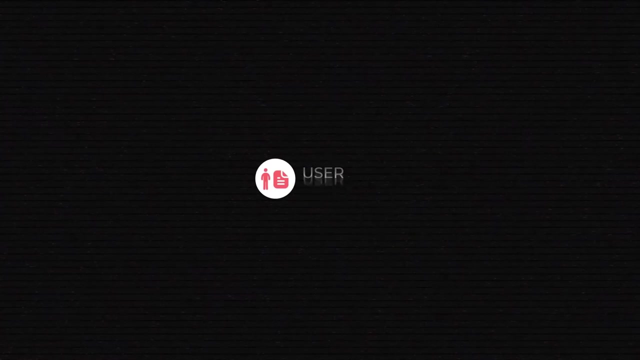 The behavior of a persona is then broken down into user scenarios about people accomplishing a task, Often represented in comic strip form. scenarios help designers understand a future user's thought process and motivation. Scenarios are broken down even further into specific user stories that look very similar. 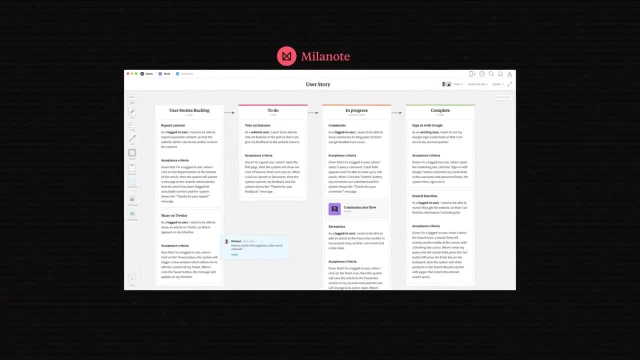 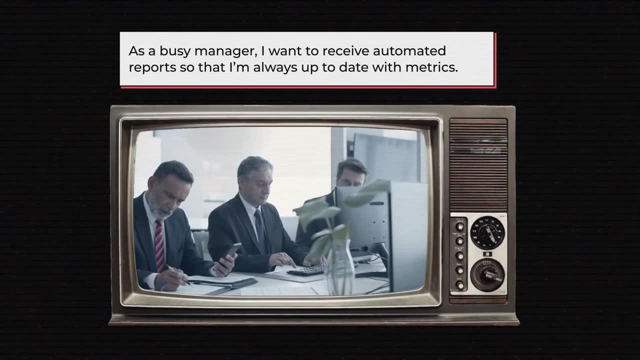 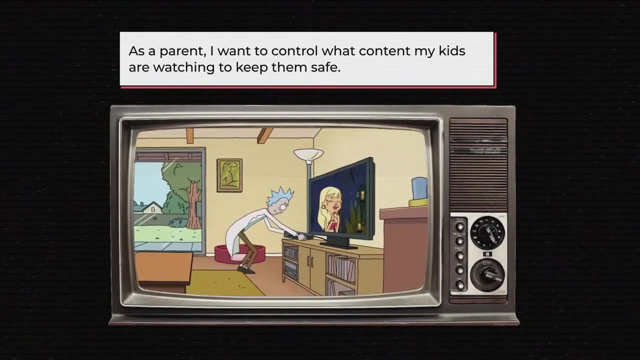 to end features. A user story is written from the point of view of a user persona and looks something like this: As a busy manager, I want to receive automated reports so that I'm always up to date with metrics. Or, As a parent, I want to control what content my kids are watching to keep them safe. 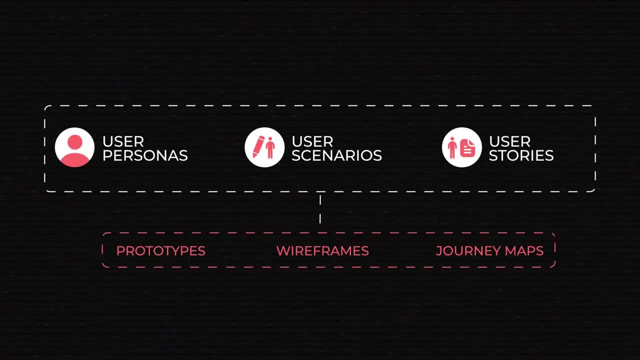 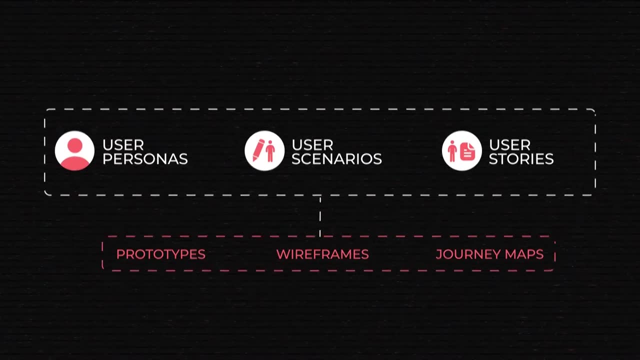 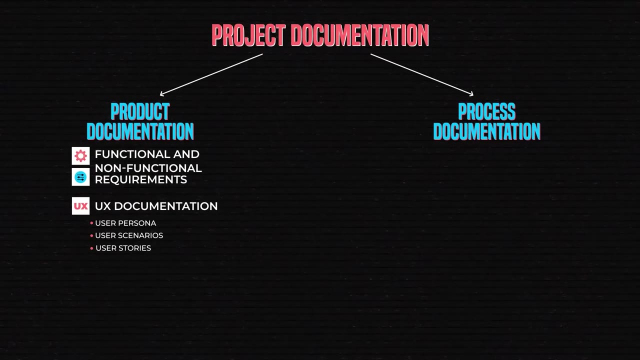 These user research docs help compile deliverables, More documentation with product prototypes, wireframes and user journey maps. These describe the future and many testing iterations later, final user experience. Okay, so we described the features and the product design. Time to talk about technology. 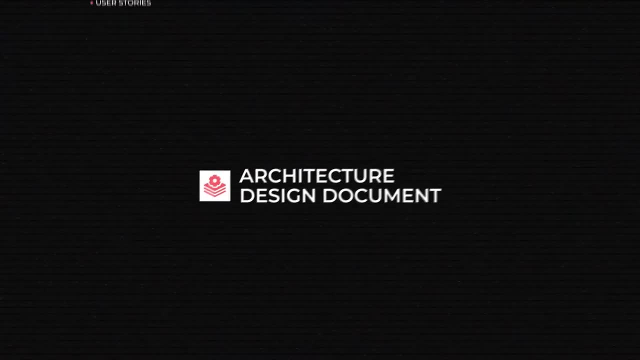 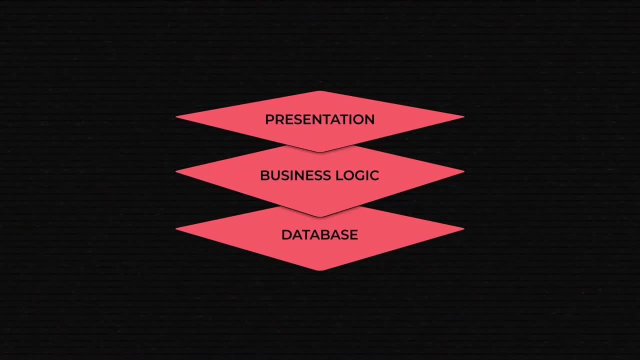 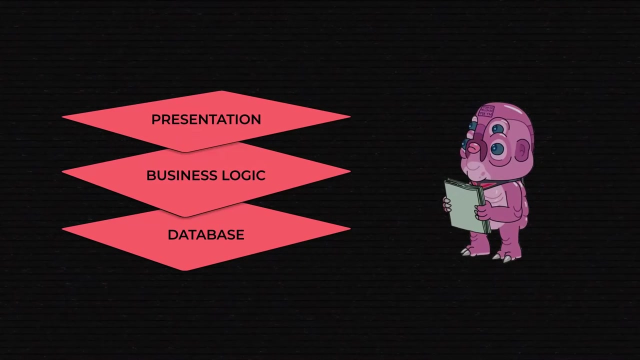 One of the first technical decisions a team has to make is a product's architecture. Although the main three architecture layers apply to most applications, many products require complex custom architectures, And these design choices are described and visualized by a software architect. Architecture depictions are usually pretty schematic, but they communicate to the team. 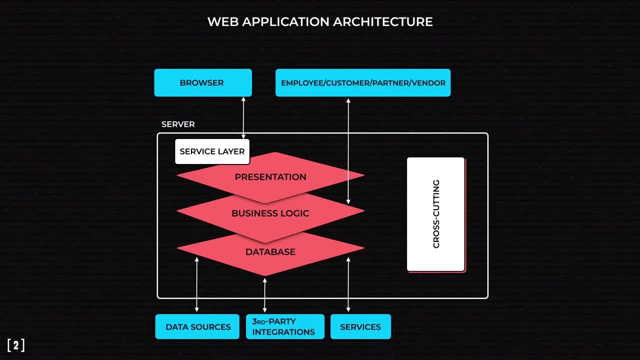 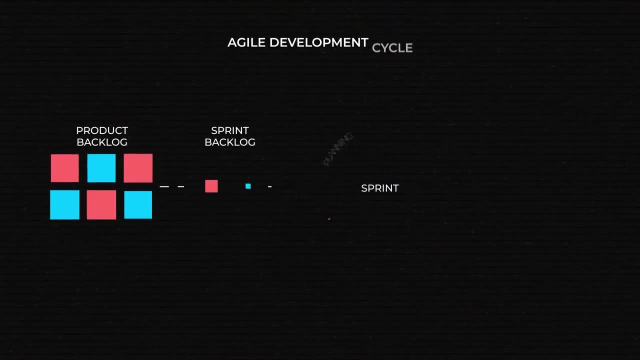 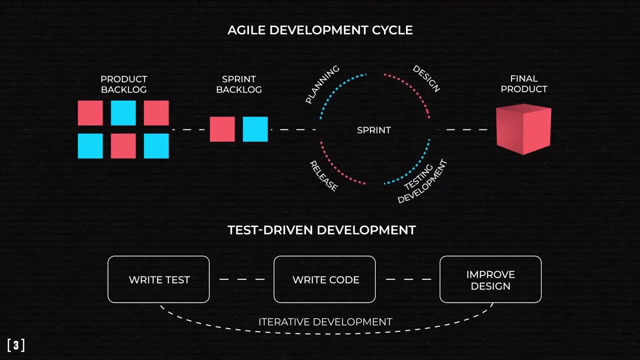 what components and design principles should be used without many tech details. What should be pretty technical is a testing plan. In agile development, testing happens along with engineering, not after, And if you're using a popular approach called test-driven development, you'd be writing. 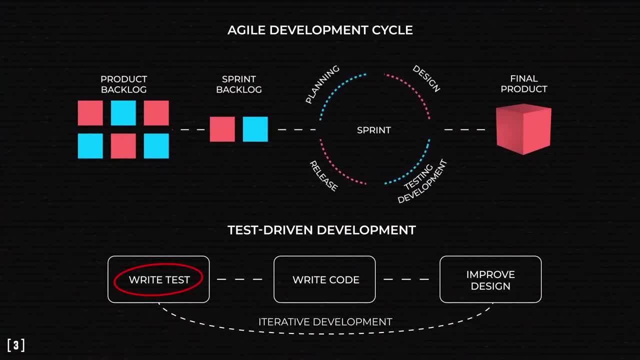 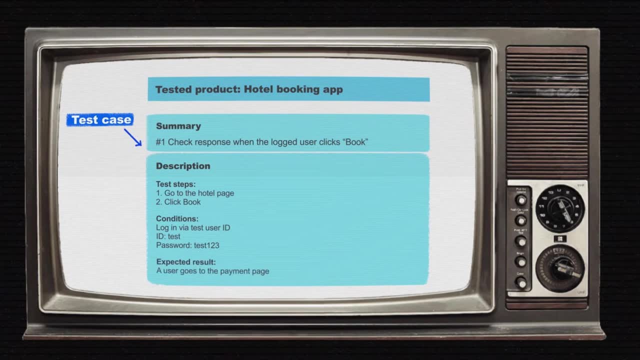 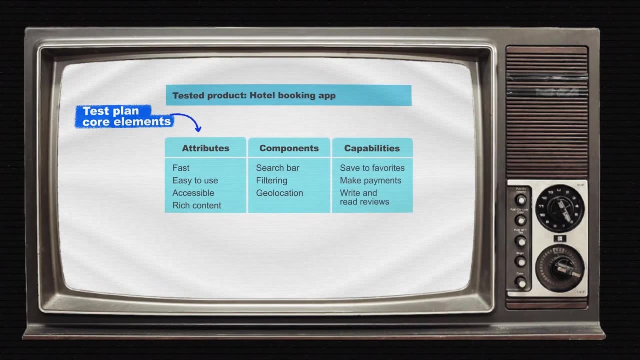 test cases based on requirements before you even start any serious development work. If you've seen our video on QA, you should know that test cases are detailed descriptions of what features should be tested and how. step by step, All test cases make up the test plan, which gives some timeframes and assigns roles to 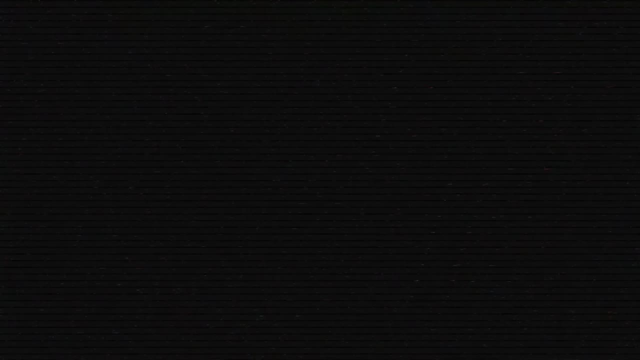 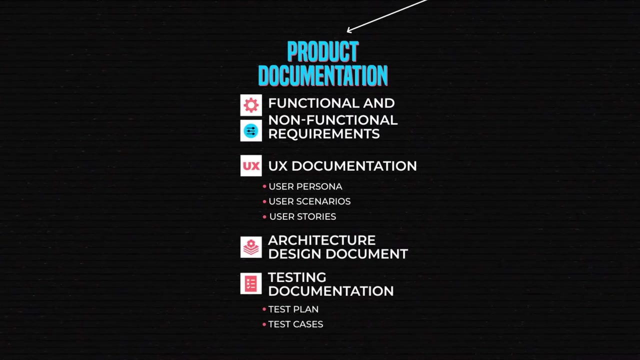 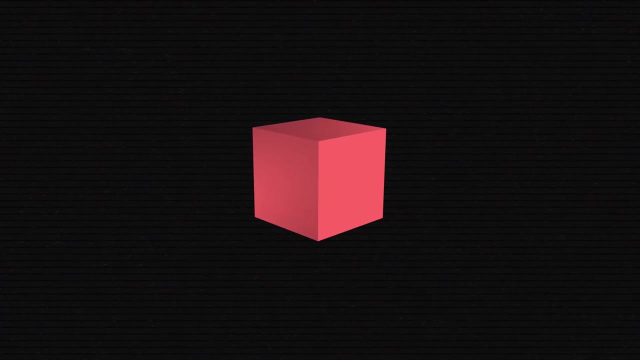 QA engineers and developers in this process. So let's recap: All this time we've been talking about product planning requirements, UX architecture and testing And testing strategy being some of the first documents created in preparation for development to tell the team what type of product they will be building. 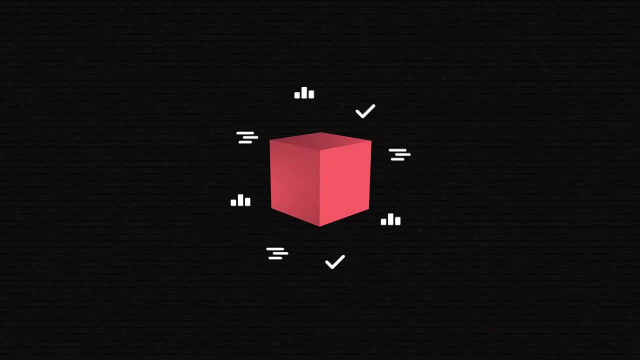 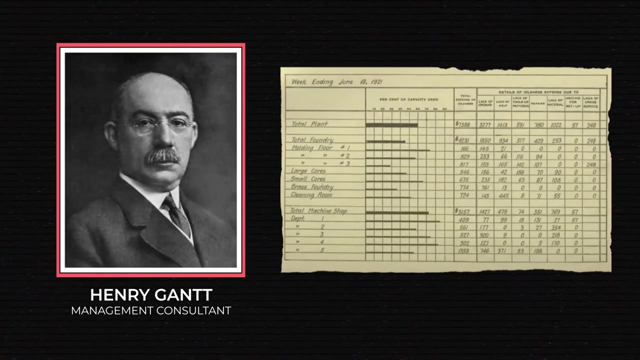 But we also need to document how it should be built, with all its processes organized around the product. Not surprisingly, this branch of work is called process documentation. The father of project management, Henry Gantt, created his famous Gantt chart more than a 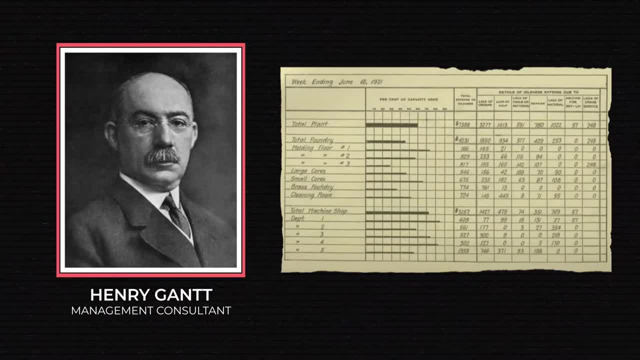 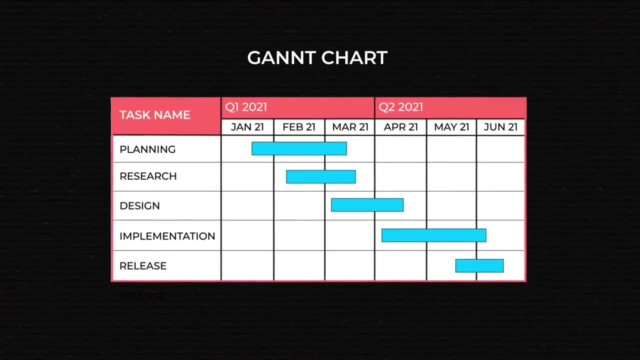 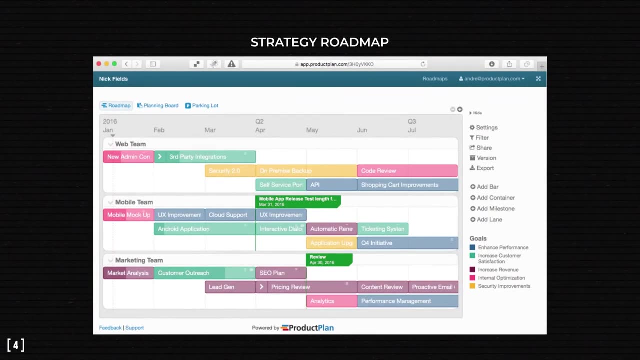 century ago And in the agile era, it's still one of our favorite planning tools. Most product roadmaps are based on the Gantt design. That's how software devs list their objectives, prioritize tasks and assign deadlines. There's a strategy roadmap with high-level goals and rough delivery estimates. 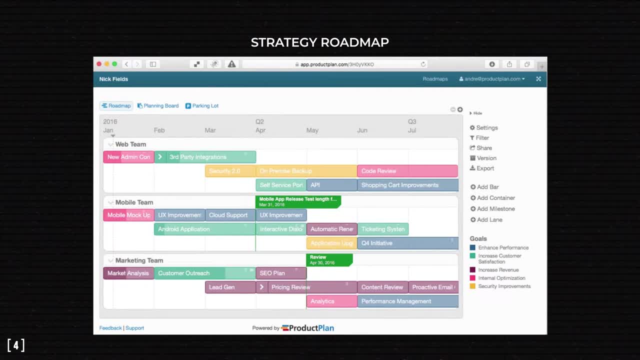 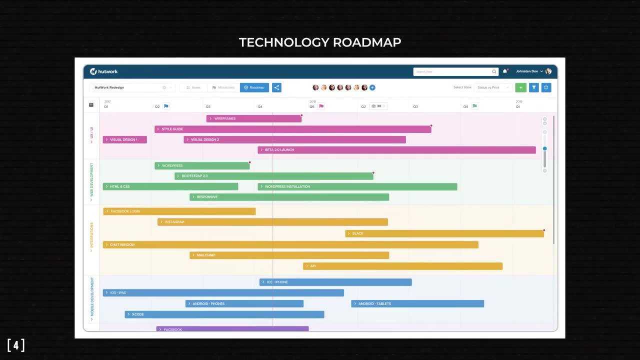 It shouldn't be detailed, because you need to view the whole project on a single screen. Then we go low-level with the technology roadmap, which lists the smallest deliverables and their due dates. Finally, a release roadmap has strict deadlines for work, And that's where Gantt comes in. 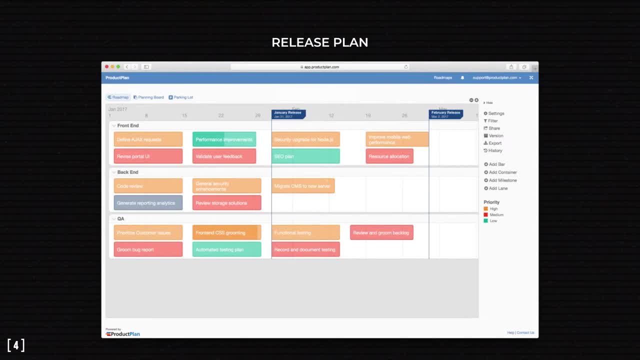 So let's get started First. let's start with the planning. The planning is a process that outlines the process and the work processes. This means you can come up with a plan to allow와 or when each part of the project should start functioning and what features go live when. 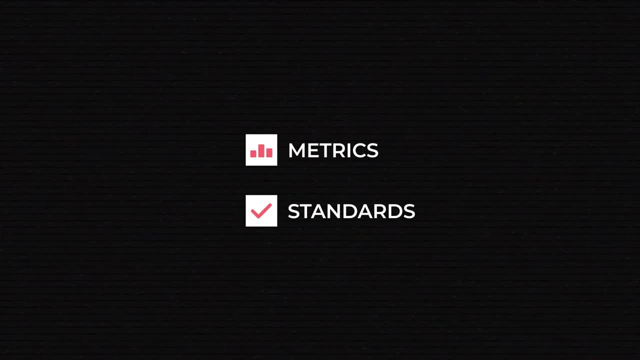 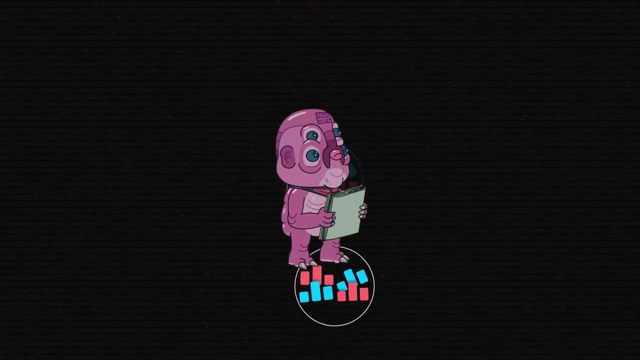 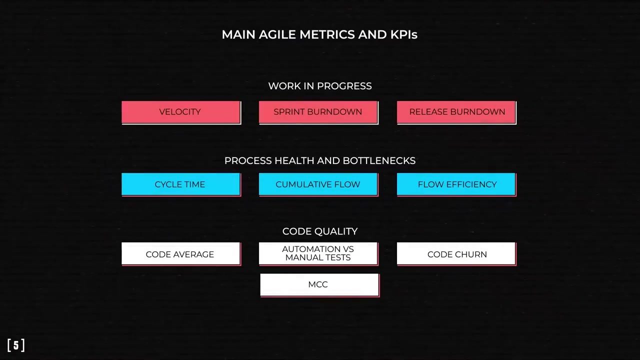 Apart from the schedule, process documentation includes metrics and standards. Project metrics are meant to provide regular feedback on how fast and effective the work is. Metrics are the main tools of the agile development process that help spot any bottlenecks and problems in the code quality before they proliferate and stall the whole project. 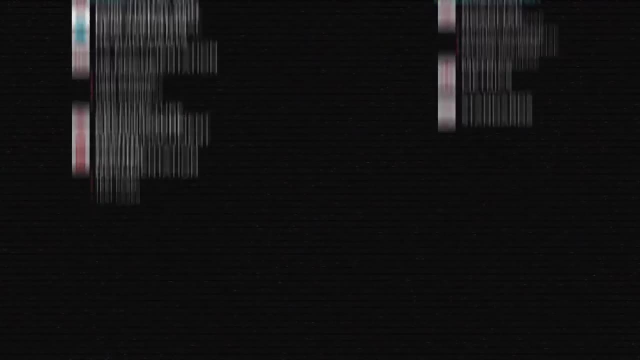 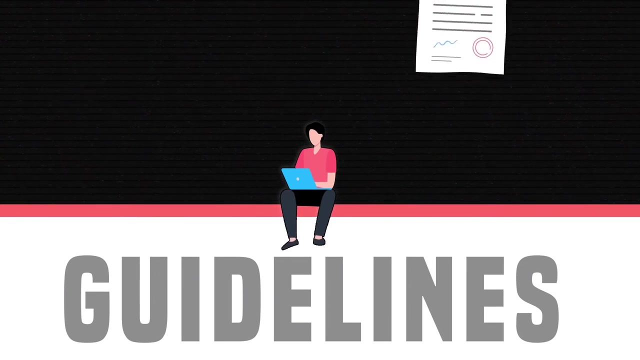 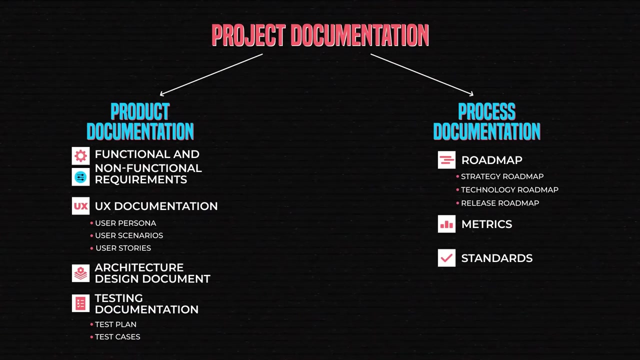 Similarly, standards and guidelines for coding and UX. people set up best practices that every team member, regardless of when they join the project or what their experience is, can use to create consistent code and design. Now you may have looked at the whole scope of document creation and wondered: